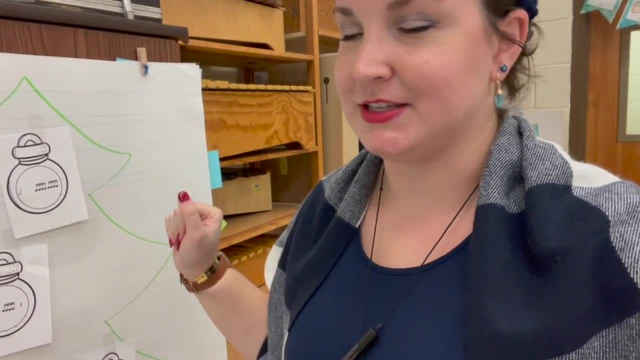 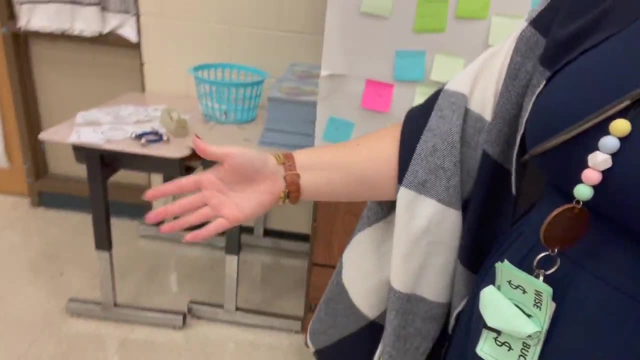 always do them in color and they would be prettier. but it's fine. Maybe I'll have the kids color them. Anyway, how you play this game is you take the ornaments and you spread them out on the floor. I just stuck them here so you can see them for now, but spread them out on the floor. I have the kids. 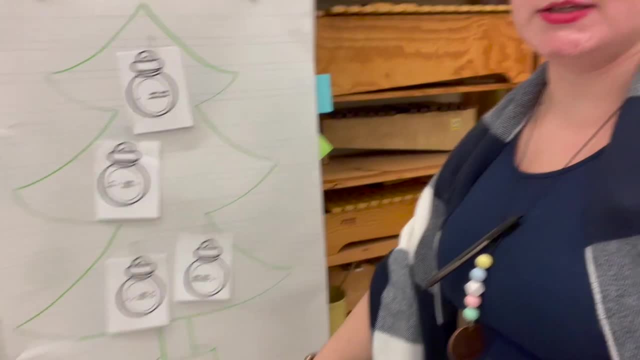 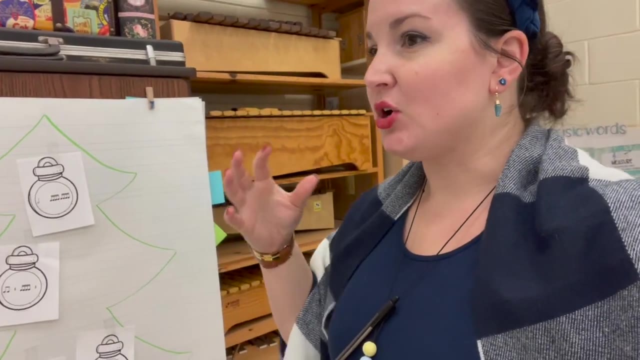 break into groups and each group gets a piece of chart paper. They make their own tree, so you don't even have to do that. or, if you're fancy, you could draw them and then laminate them. I did do this one, And so they're all in groups and they have that Now. I've already taught them the song. 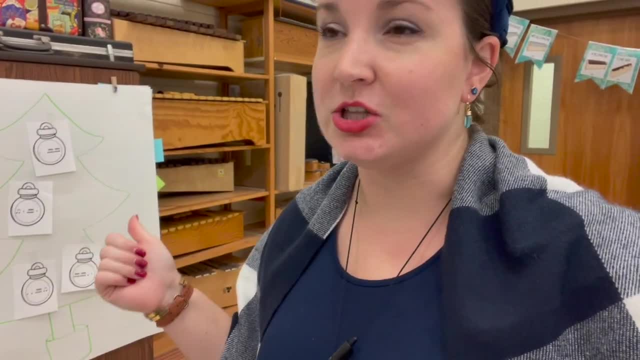 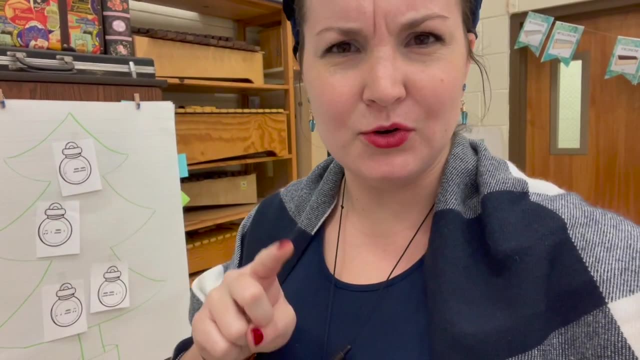 Oh Christmas Tree, because I just love that song and so we actually learn it, as O Tane and Bomb, So we really learned that song. and then this is our extension to that song. By the way, I have a free Oh Christmas Tree like lyric printable thing that you can use, and I've actually used it on my 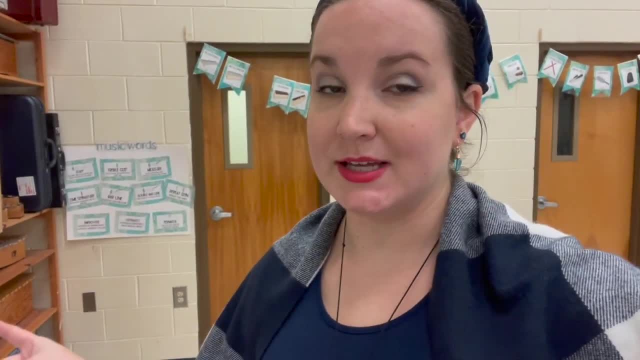 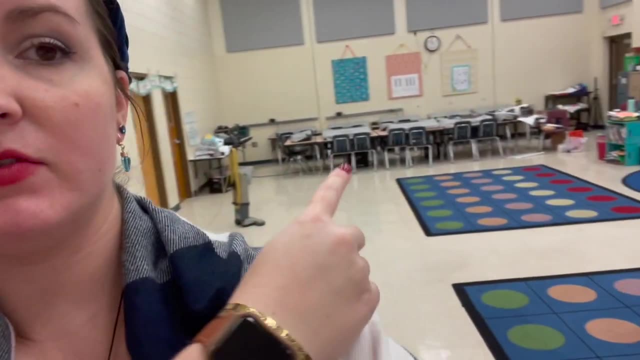 bulletin board this year and you can put up on the screen for the kids. All right, so kids have made trees. They're in groups. The next thing we do is one person lines up in a designated spot, So one person of each group lines up. i have them line up on this edge of the carpet. no, that clock's. 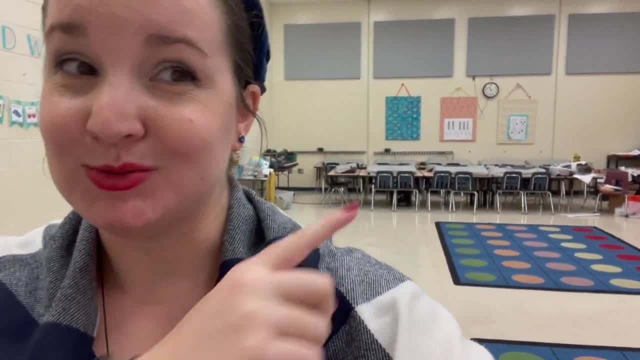 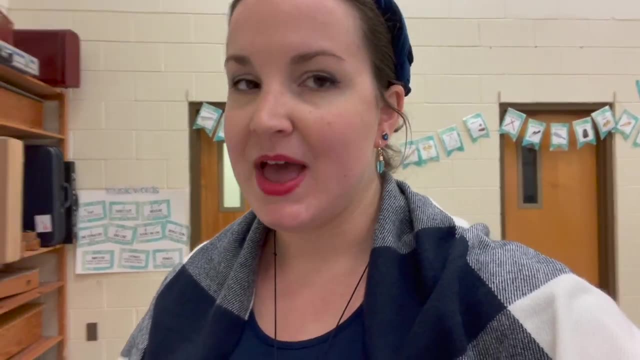 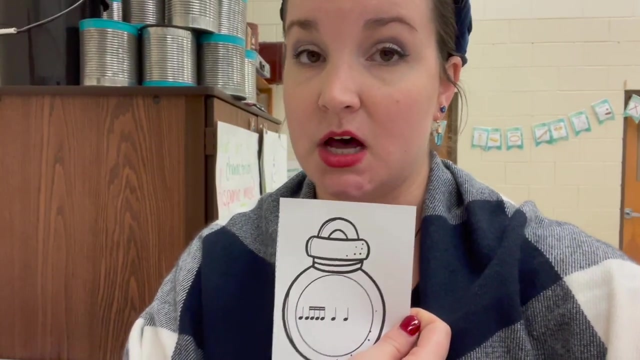 not right and sorry for the giant mess. um, it is after school, but they line up on this side of the carpet and we all sing the song: oh christmas cheer, oh tan and bomb. at the end of the song i read out one of the rhythms. so if i do ta tikka, tikka, ta ta, then once i read the rhythm, you can't move till. 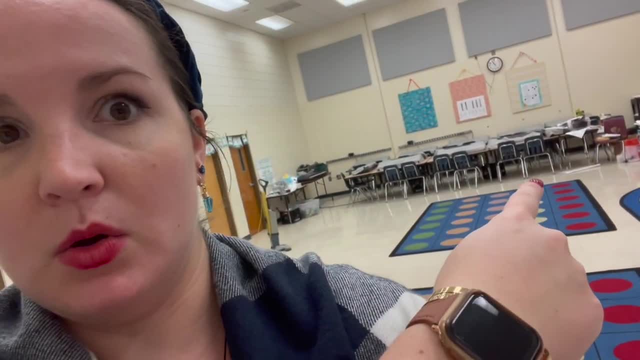 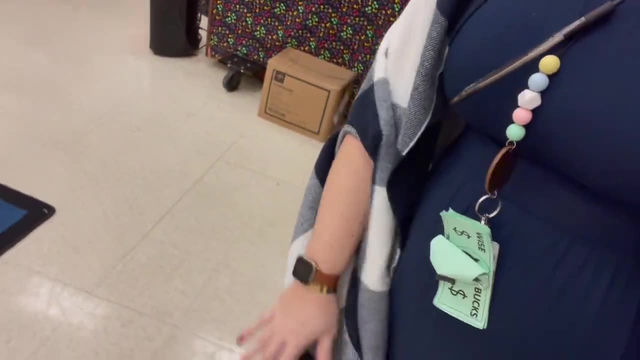 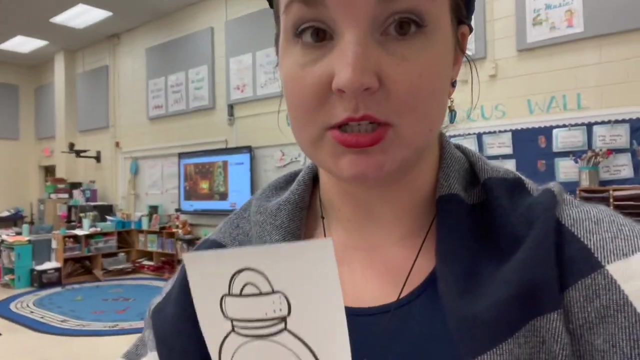 i read the rhythm. when i read the rhythm, then the kids at this end walk carefully so they don't fall and hurt themselves down the carpets, and i usually have them all over the floor right here and they have to find the correct rhythm. whoever finds it first wins a point for their team, so they 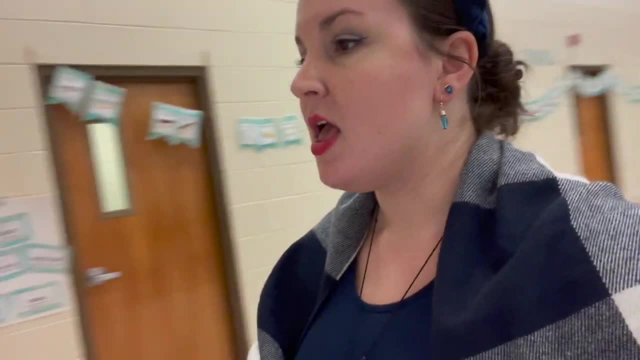 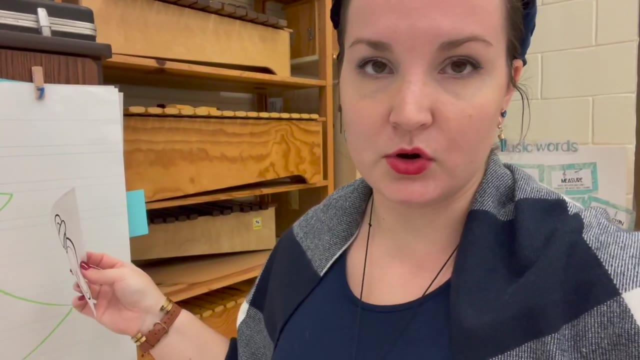 get to take the ornament back and put it on their tree. now you can do this with the trees on the floor. if you laminate them, then you can hang them up, or you can hang them up like i did and tape them up. whichever way you want to do it. 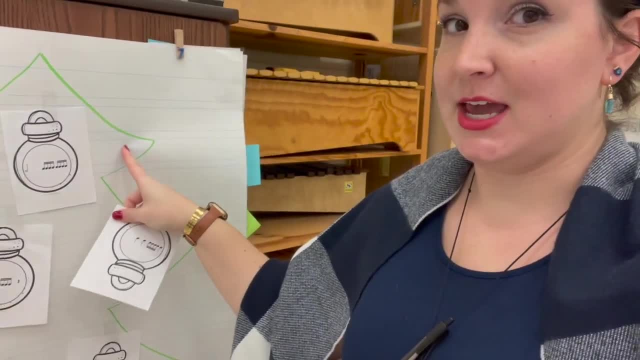 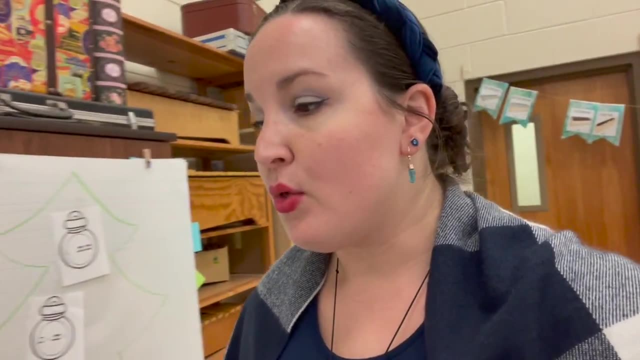 but i will say i actually would prefer not to do it like this way because i can't move these around. the reason is at the end of the game, once we've gotten lots of ornaments, somebody has won. then the kids take the ornaments that they have gathered and they arrange them on the christmas.